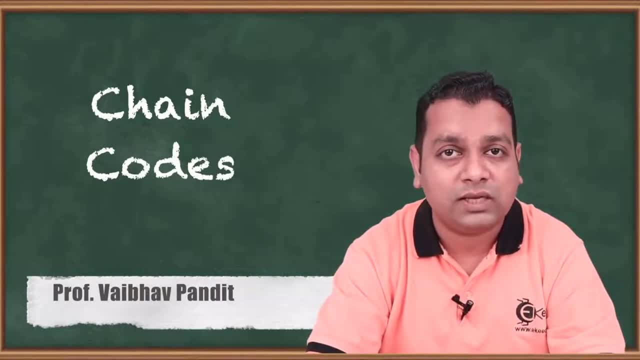 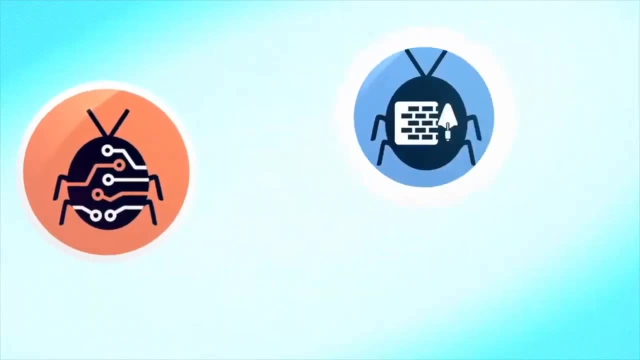 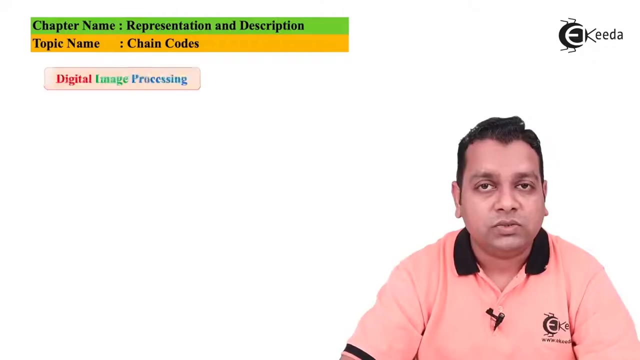 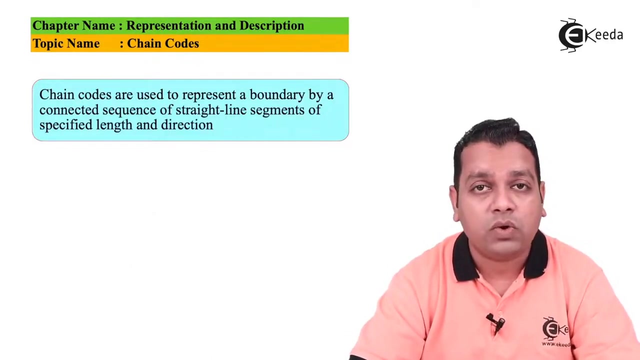 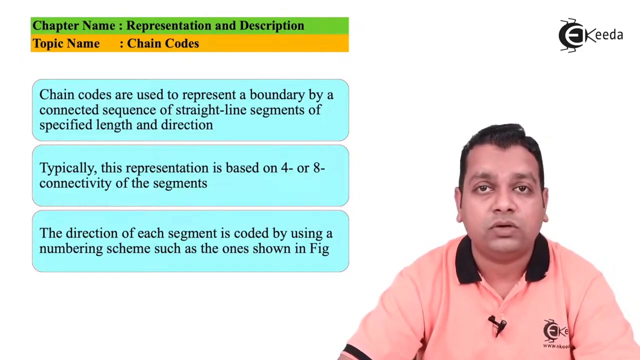 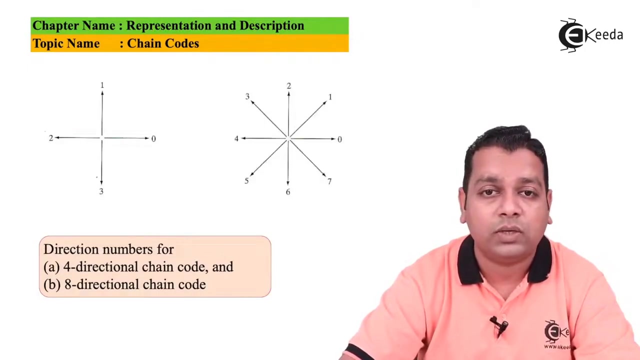 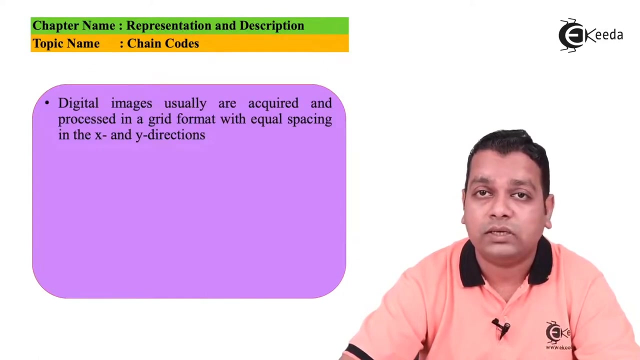 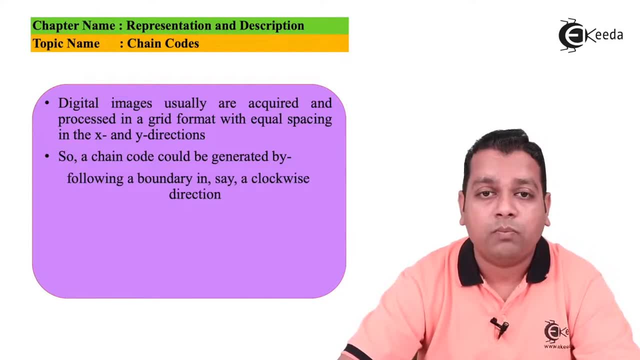 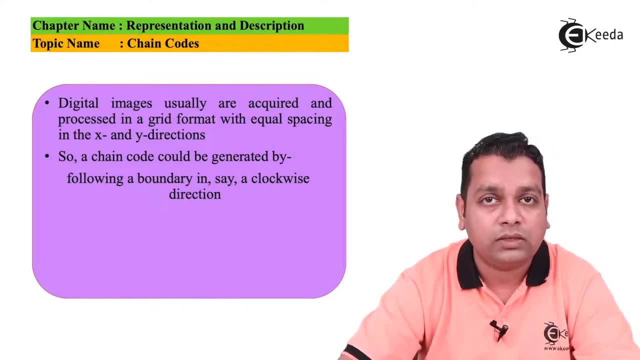 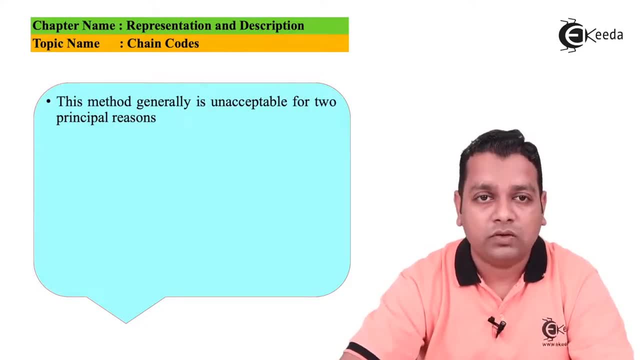 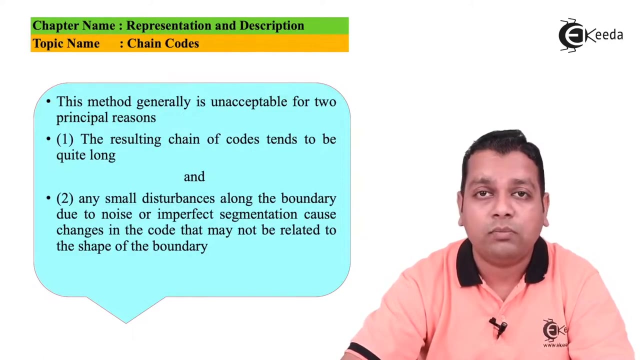 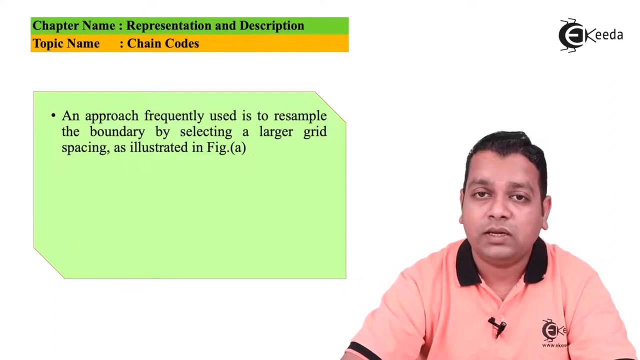 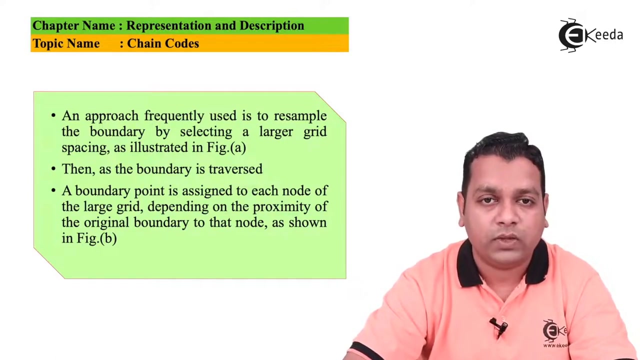 for the two principal reasons. The first reason we can give the resulting chain of codes actually tend to be quite very very long and the second reason is that any small disturbances along the boundary due to the presence of the noise or imperfect segmentation technique if it is opted onto the original image causes the changes into the code that may not be related to the shape of the boundary. An approach frequently used is to resample the boundary by selecting the larger grid spacing that can be illustrated into the figure A. Then the boundary is traversed. A boundary point is assigned to each and every node there of the larger grid depending on to the proximity of the original boundary to that particular node as shown into the next figure B here. So here we visualize both the figures. The captions are here. 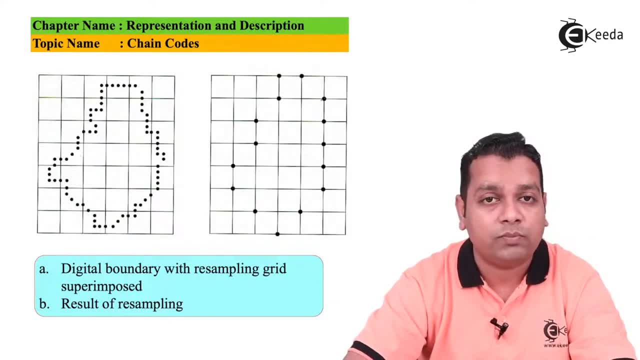 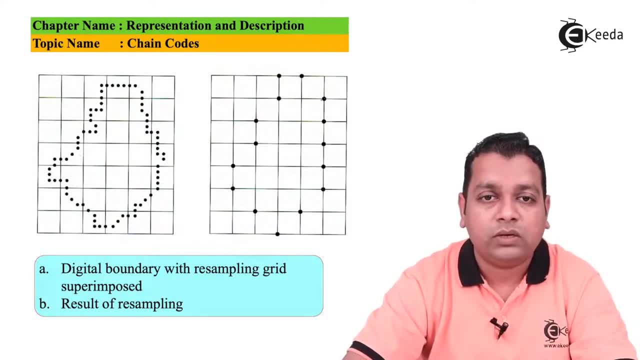 hand side. That is the result of resampling. So here on the left most image you find lot many black dots because of resampling of the grid superimposed onto the image sample. The representation of the 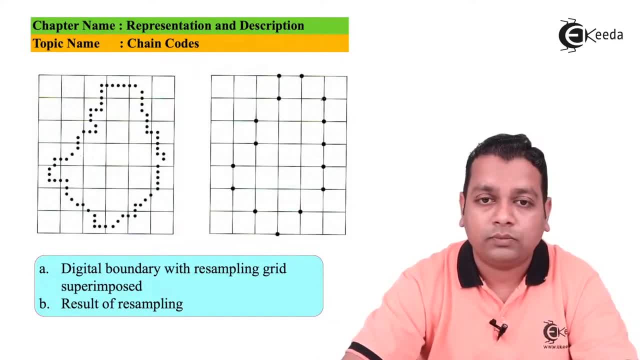 digital boundary here we have. And after resampling of the grid superimposed onto the image sample resampling we have only few corners into the grid represented with the dark dots here. The 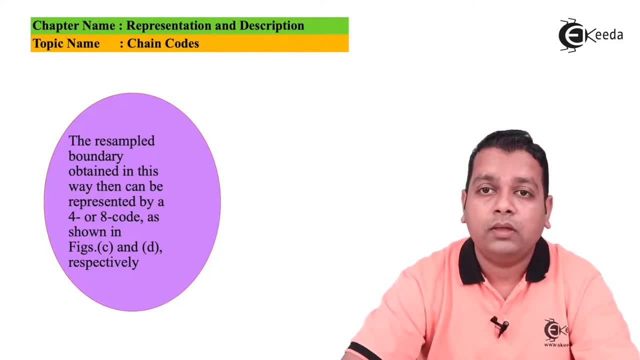 resampled boundary thus obtained into the figure B we can be represented by the four or eight connectivity chain code as shown into the next figures that is figure C and figure D respectively. 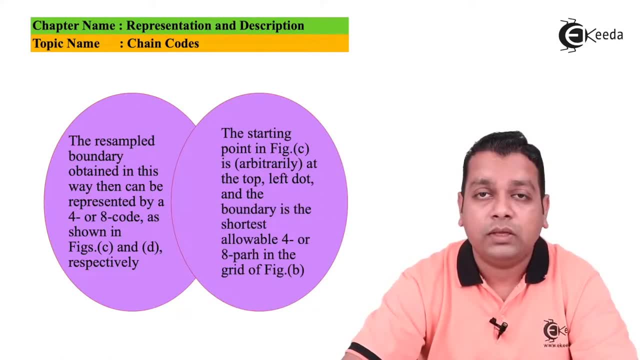 The starting point into the next figure C is actually the arbitrary selection at the top left dot and the boundary is the shortest allowable four or eight connectivity path into the grid of 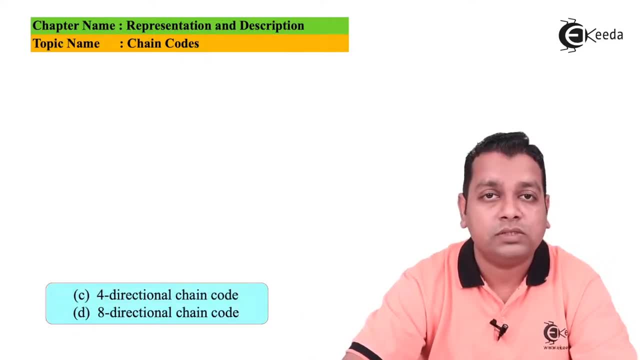 figure B. So here we have the visualization of figure C and figure D. So this is figure C 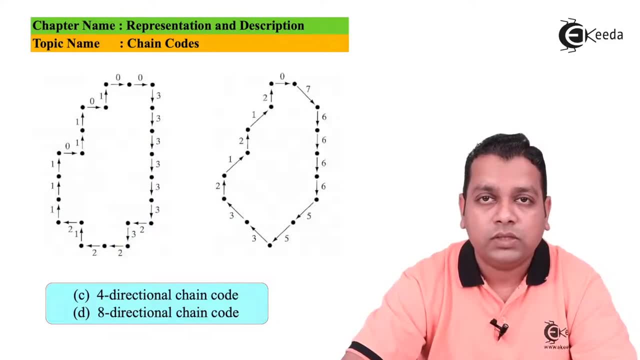 representing the four directional chain code. So at the left hand side and the top corner here we can start. Then we have as per the pattern we have seen for the four connectivity we are going towards the right hand side. Hence the first 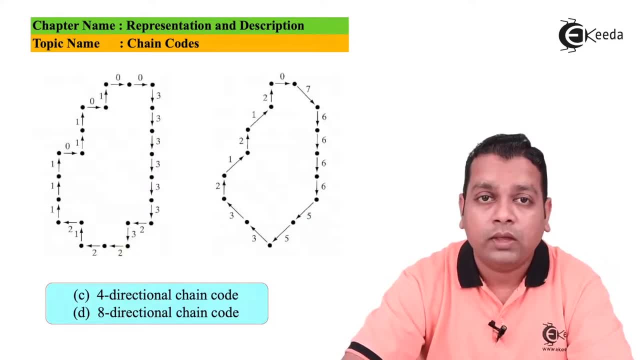 digit into the chain code shall be equal to zero. Then again we have the same direction to follow so 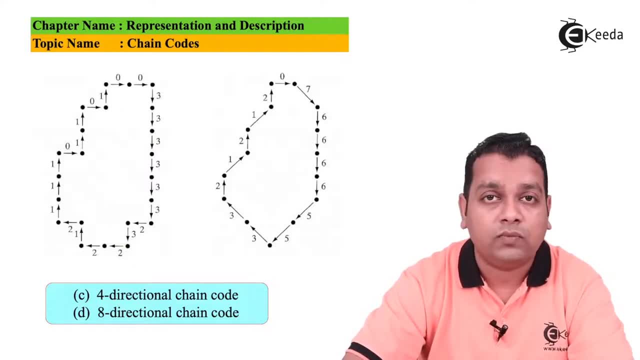 it will be again the second digit to be the zero again. Then we are going downwards so we shall be having the representation of this direction by the number three here. So we can find the three 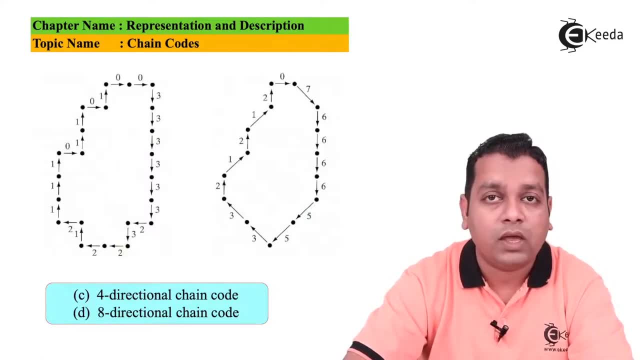 number repeated for six nodes here. Then we have the direction towards the left hand side representing 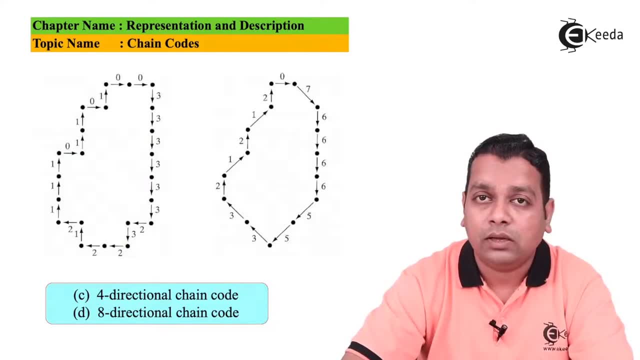 we have three then we have two times the left direction representing the digit two then one two 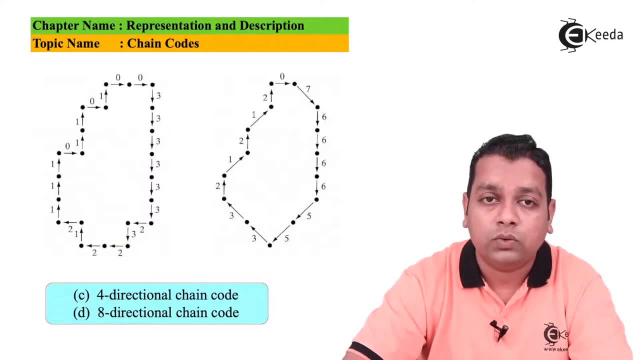 one one one into the upward direction then zero one one zero one completes the sequence here and 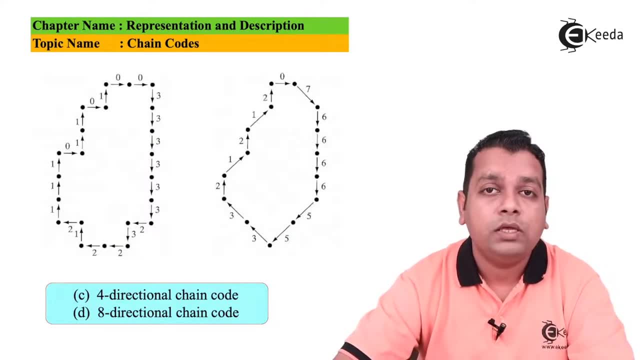 we come back to the original point here now if you take the case of eight directional chain code 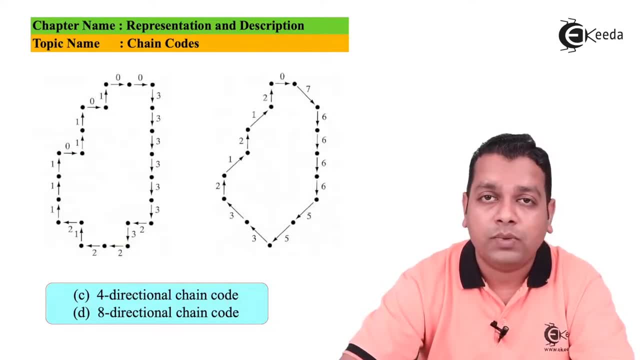 some efforts in representation of the chain code will be minimized here the representation will be 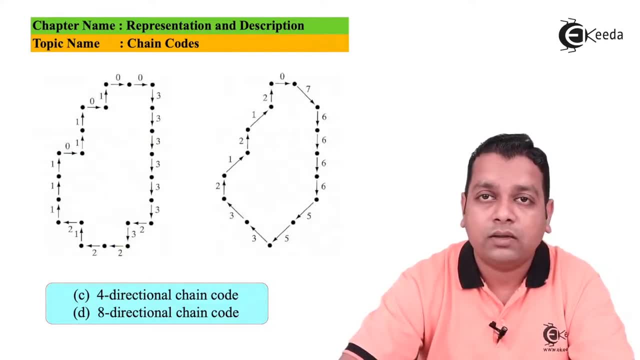 somewhat shorter here so we again start at the top left corner there that has this representation 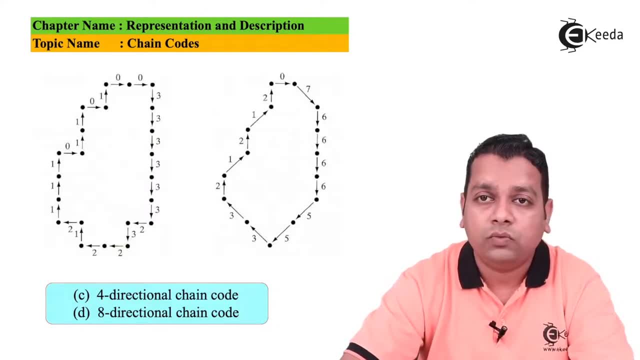 and starting with zero here so after this zero we can go with the representation of the digit seven 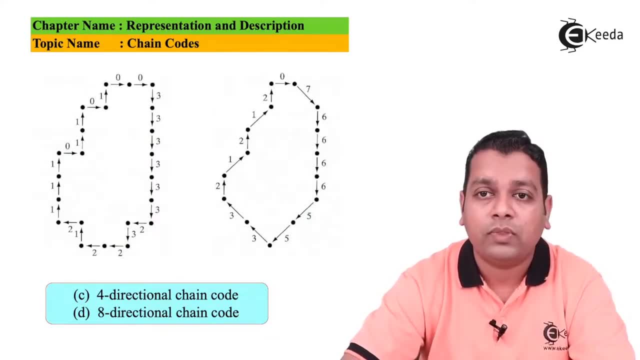 for this chain code as it is available with the eight connectivity then we have four times six 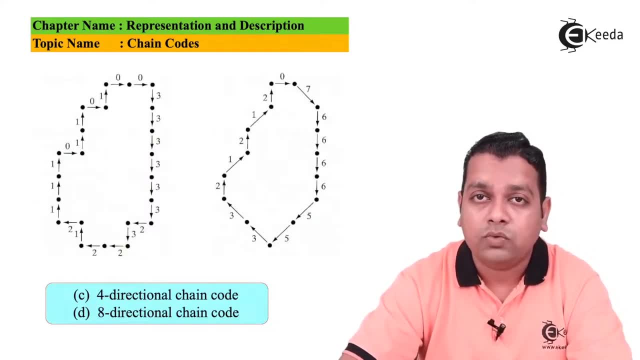 representing the downward direction then we have piu representing the south west direction two times then we have the two 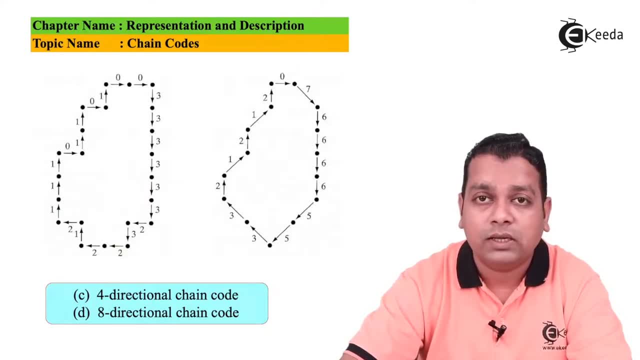 times three representing the north west directions then the upward direction can be represented here 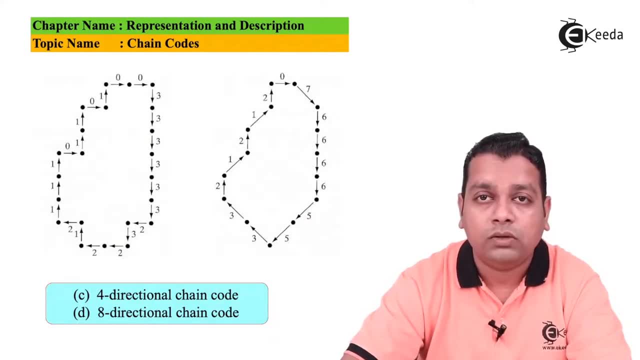 by the digit two then we have one two one two and we are back to the original position now the 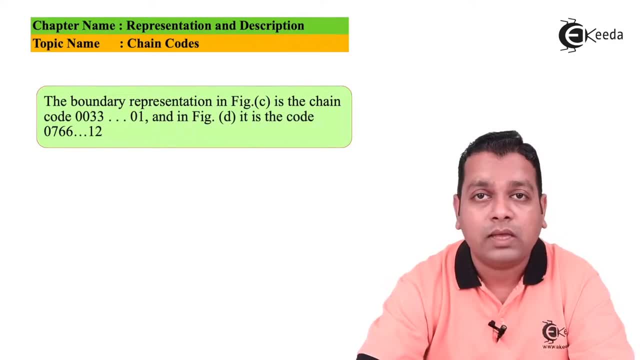 boundary representation that we have seen into the figure c as the chain code we can write as 0 0 3 3 and so on up till we get back to the original place with 0 1 here and into the right hand side we have seen the figure d 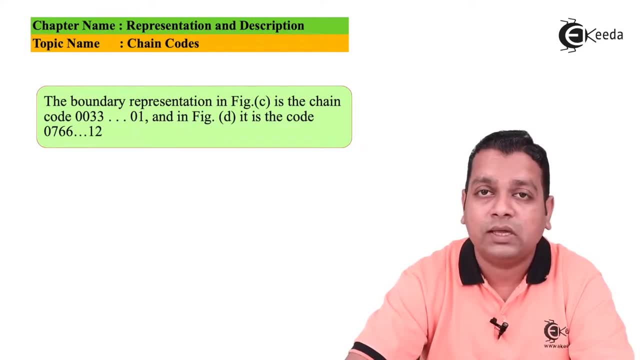 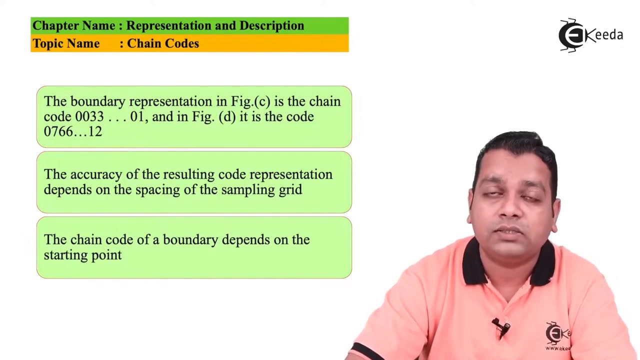 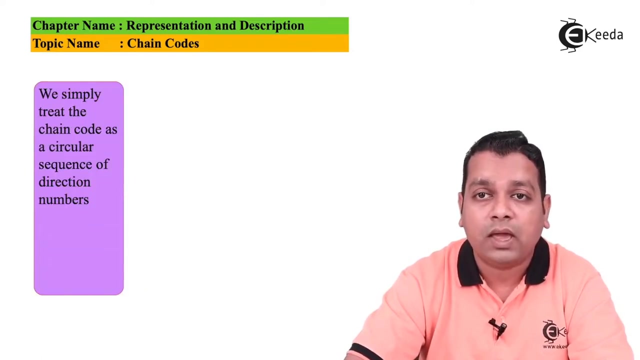 the chain code can be represented as 0 7 6 6 as like we can come back to the original place with 1 2 at last here so the accuracy of this resulting code representation actually depends onto the spacing of the sampling grid provided earlier the chain word of the boundary actually depends onto the starting point so we had selected the starting point at the top left corner as arbitrary manner now here we can see that the chain code can be represented as 0 7 6 6 as like we can come back to the original position here we simply treat the chain code as a circular sequence of the directional 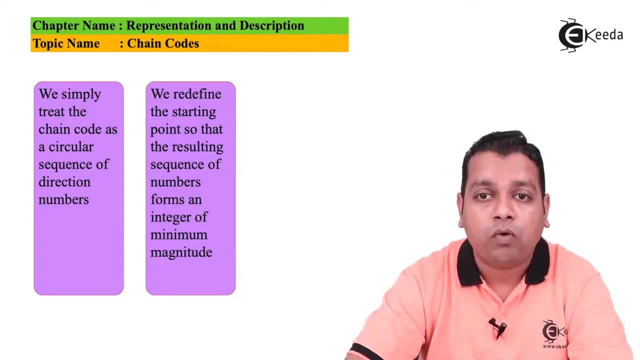 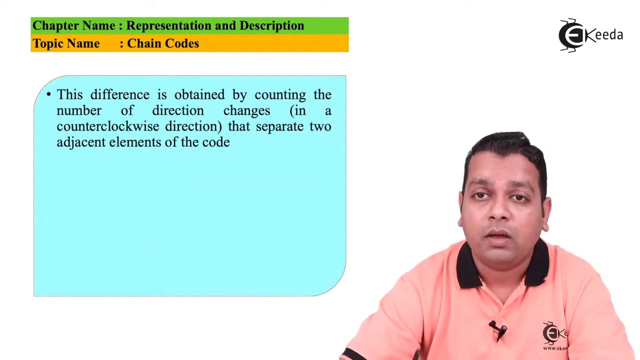 numbers we redefine the starting point so that the resulting sequence of number forms an integer of minimum magnitude we can also normalize for the rotation by using the first difference into the chain code instead of the code itself now this difference is obtained by counting the number of directional changes that is into the counterclockwise direction that is separates two adjacent elements of this chain code now for instance we can take the first difference of the four directional chain code represented as